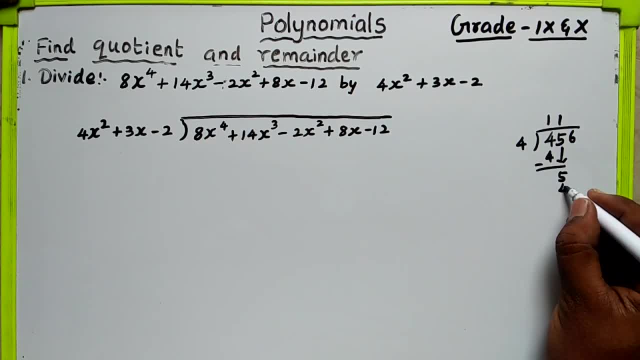 5 and again one time 1 into 4, 4.. Here remainder is 1.. Next we will take 6 and 4 forcer 16.. So always we will try to make the value is 0 or less than that. The same way we will. 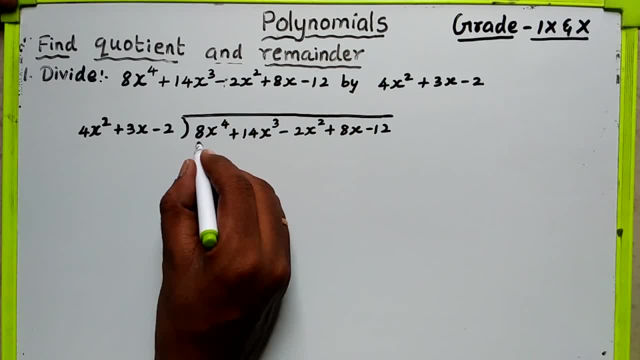 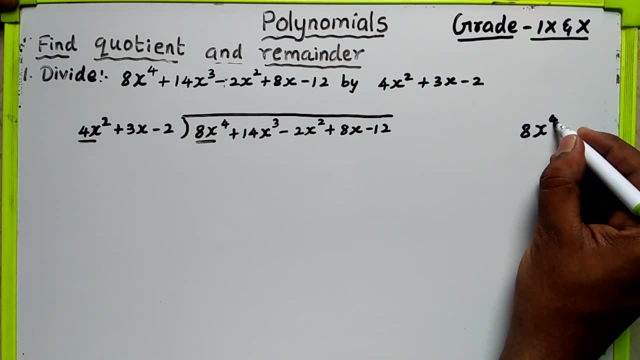 solve Here. the value is 8x power 4.. Divide 4x square 8x power 4. divide 4x square 4, 2 times 8.. Here x power 4.. If we cancel here x power: 2. Using loss of exponent x power 4 by x power 2, x power 4 minus 2, x. 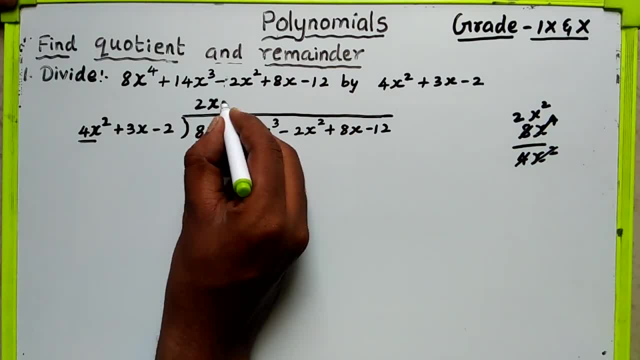 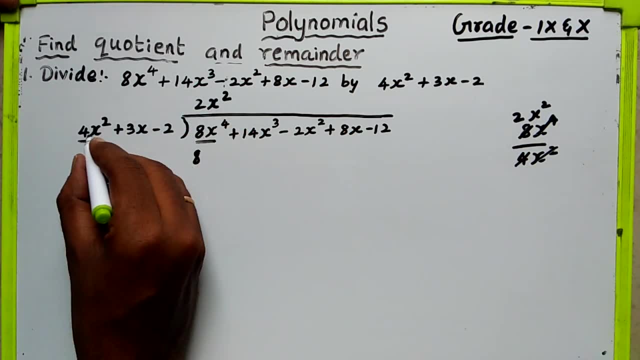 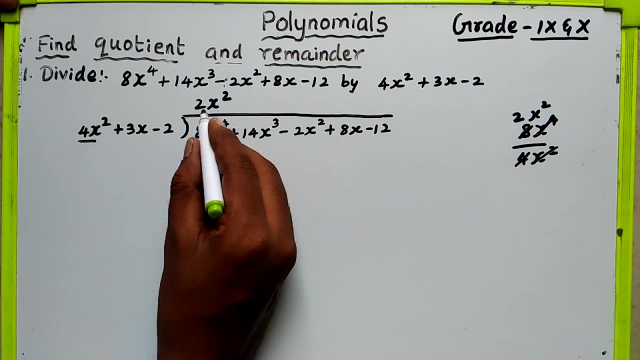 power. 2. The value right here: 2x square. Now you multiply here 2 into 4, 8x square x power 4. Plus into plus, plus 2 into 3, 6. And x square into x. x power 3. When base. 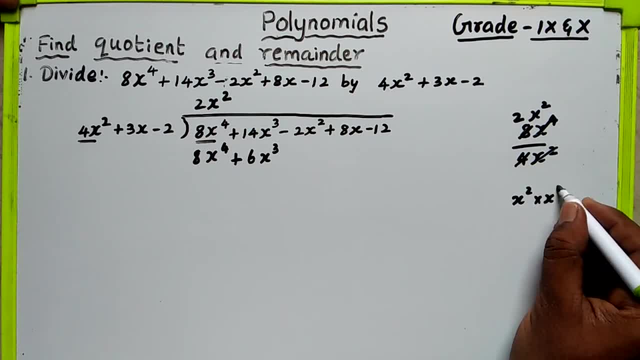 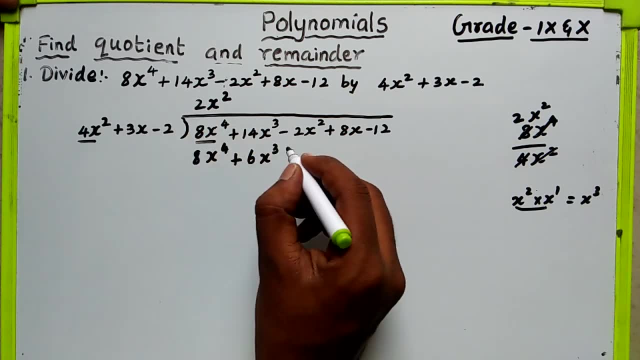 are same. we have to add the power, x power 2 into x, power 1, x power 3. Base are same. We should add the power And plus into minus, minus, 2 into 2, 4.. Here x square, So we will. 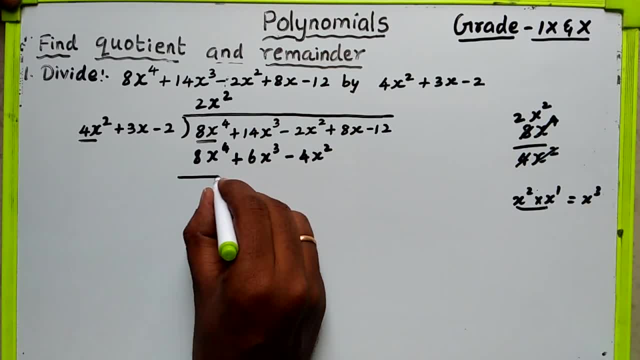 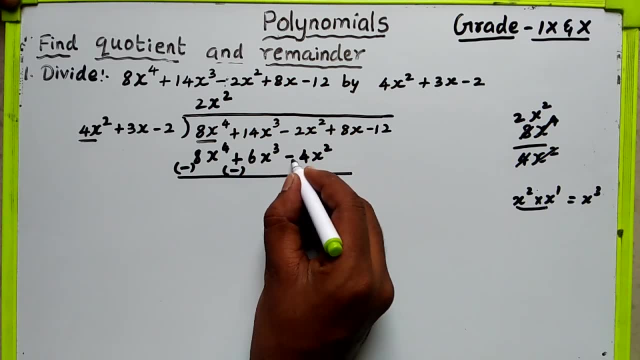 write here directly: x square. We will change the symbol. We will do: subtract Plus 8 change minus 8.. Plus 6 change minus 6. here, Minus 4 change plus 4.. 8x power 4, minus 8x power 4, cancel. 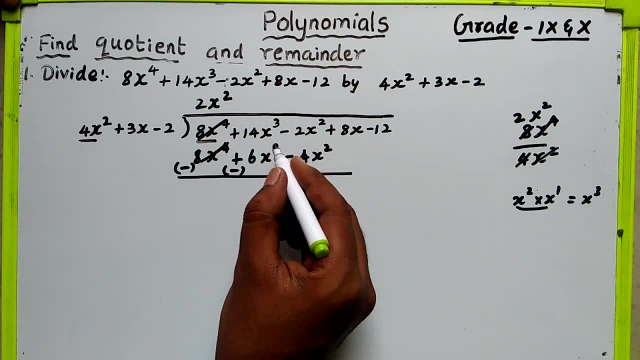 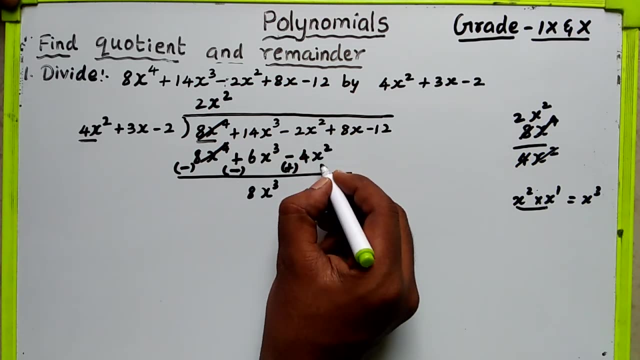 And 14x power 3, minus 6x power 3.. Write the variable first: x power 3,. same variable: 14 minus 6 is 8.. The same way, first way you write the variable here: x square And minus 2 plus 4 is plus. 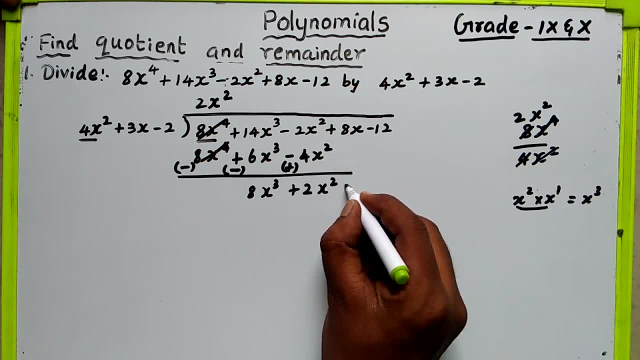 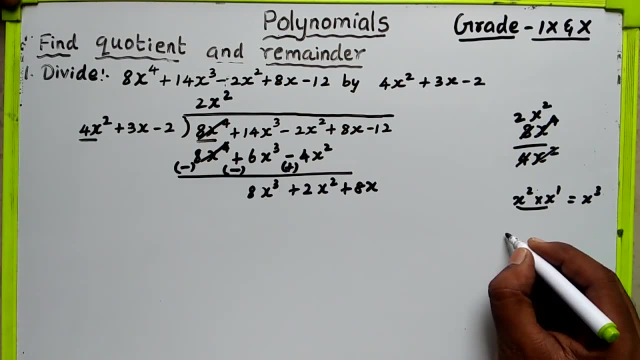 2. 2x square And take the next term, 8x. Now we need here 8x power 3.. Here we have 4x square. Do the as usual division: 8x power 3, divide 4x square If we cancel here 2 times. we will get 8x power 3. And here we have 4x power 3. And here we have 4x power 3. And here we have 4x 5.. And here we have 2x power 3. And here we have 4x 5.. And here, since we 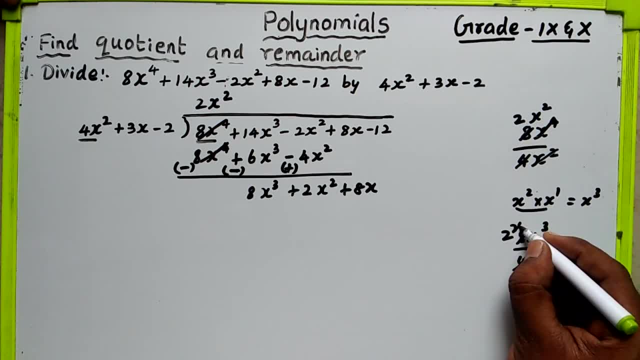 have 4x, 2x, So both sides in sides. So plus 5, plus 4,, minus 6x power 3, so that'll get X power 3. And so 2x power 3. And so now 2 is 8. So we will add 10x power 3.. developments: 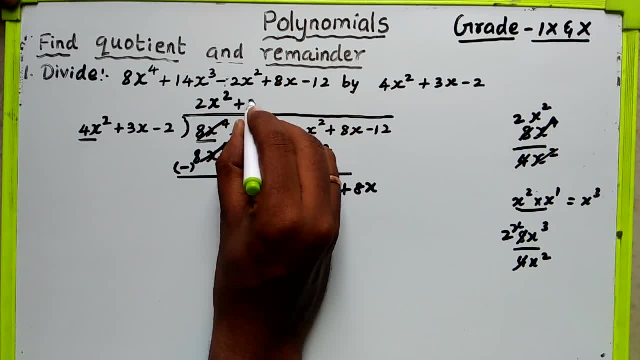 will be a new factor brother. So x power 3, and 8. I'll obtain 2x power 2.. I'll use 7x power 3.. So now I'll take this 2x really, but 10x power 3. And I need x to be equal to 141.. So here'll make. 10x power 3.. So if you multiply that by 14.. So here this: 1X power 3 plus 1, I'll get 8x power 3 minus 8x power 2. And x divided X power 2 will get X power 1, 2x. Write the. 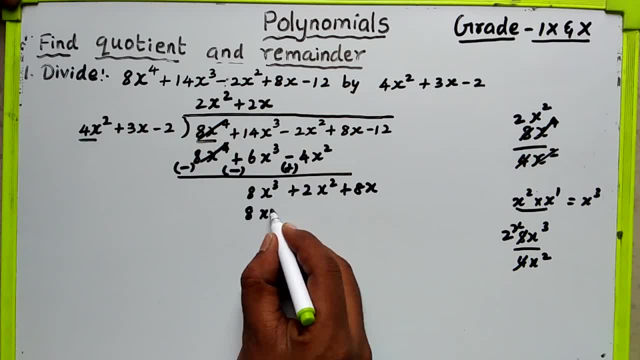 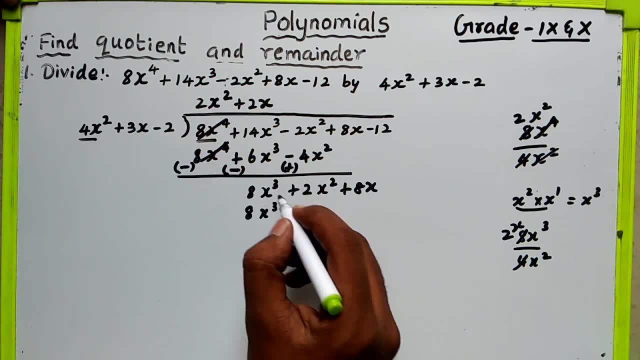 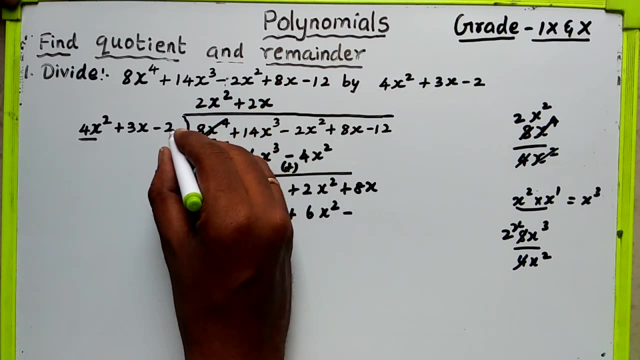 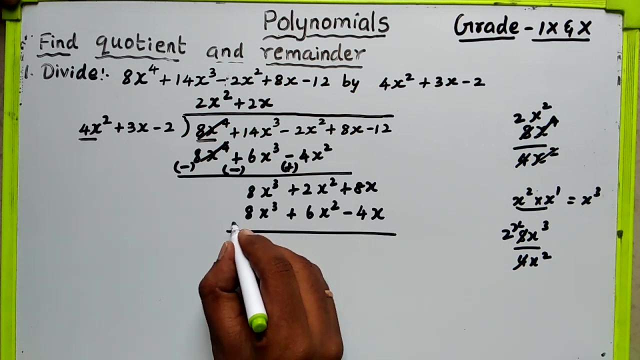 4, 8, and x into x. square x power. 3, and plus into plus plus and 2 into 3, 6,. x into x. x. square plus into minus minus 2 into 2,, 4, and x 4x. Change the symbol subtract. 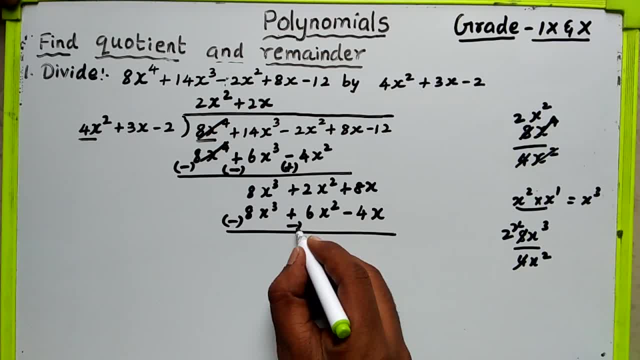 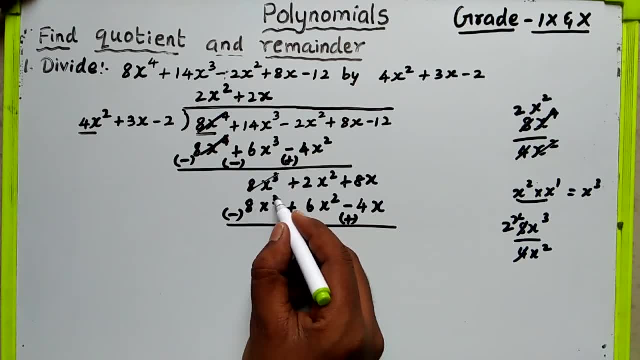 plus 8x, change minus, 8x cube. and plus change, minus and minus, change plus. Now cancel it. 8x power 3, 8x power 3, cancel and x square. bring the variable here and plus. 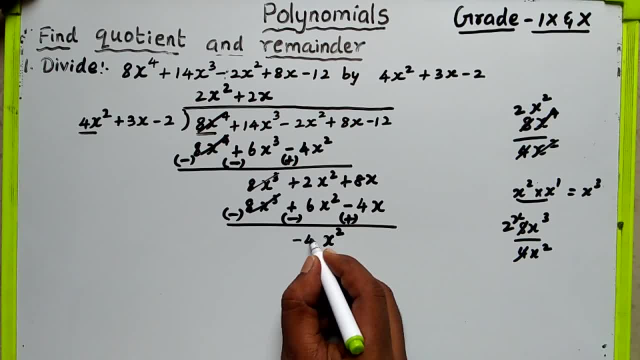 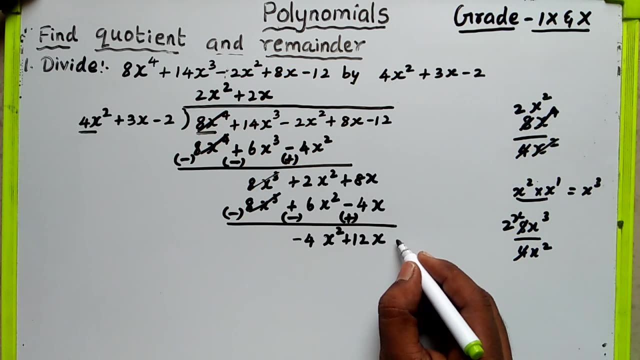 2, minus 6, plus 2, minus 6,, 6, minus 4, minus 4, and x variable is x and 8, plus 8, and plus 4 is plus 12.. And take the next term here: minus 12,, minus 12.. 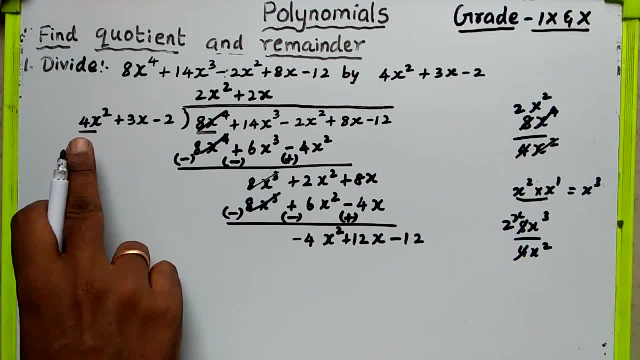 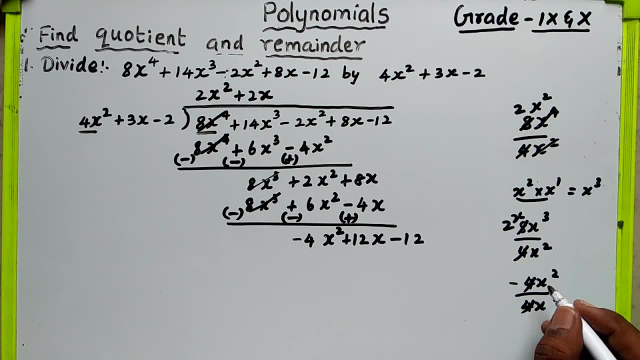 Next, here we have minus 4x square. here plus 4x square, minus 4x square divided by plus 4 x square: 4- cancel one time. and x square: cancel one time Your minus symbol. we need minus one. 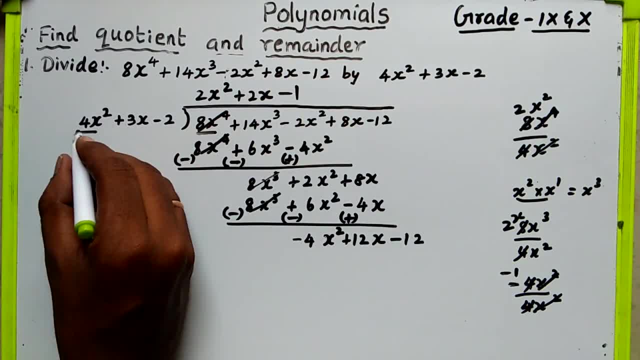 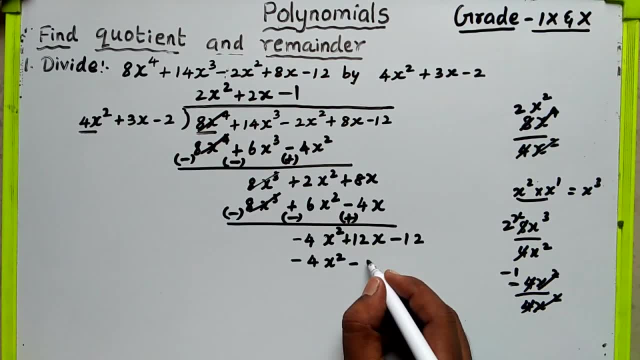 In the portion plays your right minus one. So minus one into 4x square, minus 4x square and minus 4x square x square. minus into plus, minus one into three, three x and minus into minus plus one into two, two.